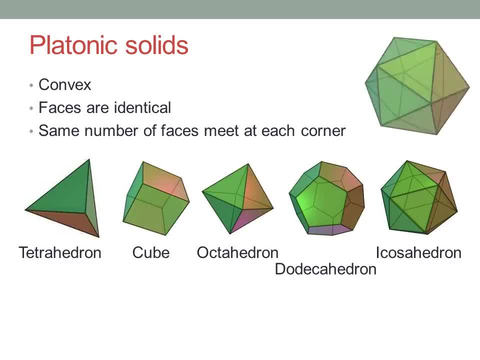 Dodeca means two and ten, And the icosahedron again has triangular faces, 20 of them. The tetrahedron has three triangles meeting at each vertex, the octahedron four and the icosahedron five. 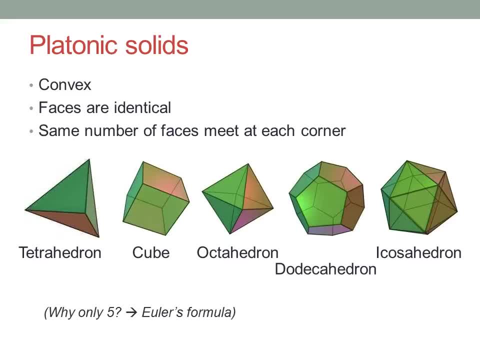 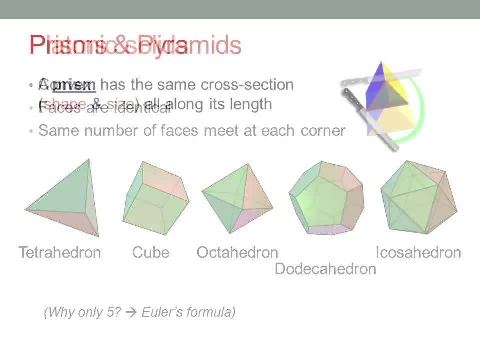 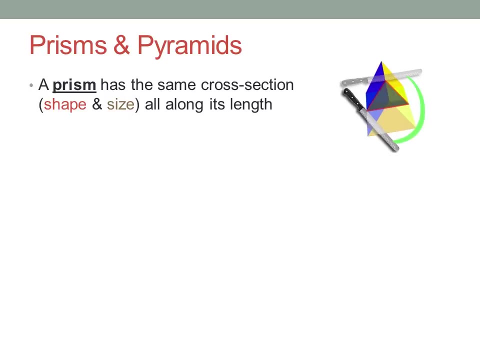 Can you work out why there are only five platonic solids? Look up Euler's formula and see if you can prove it to yourself. A prism is a solid shape with a flat base that keeps the same cross-section all the way through its length. 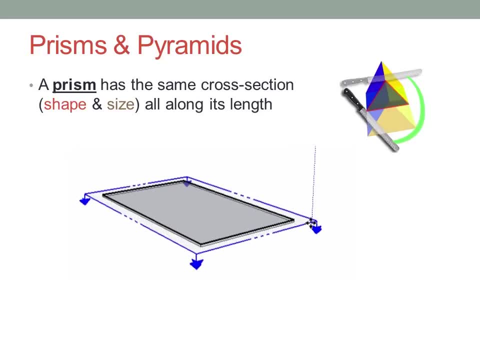 If you take a cross-section parallel to the base, wherever you are, and you look along the prism, you'll see exactly the same shape and size all the way along. Be careful, though: The base may not actually be on the bottom. 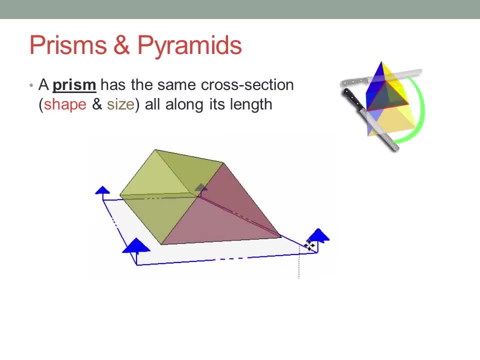 In this prism. if I try to use the bottom surface, I'll get a rectangular cross-section that gradually reduces in width, but not length, until it becomes a line at the top. But if instead I use the triangular end, look what happens: It's the same triangle all the way along. 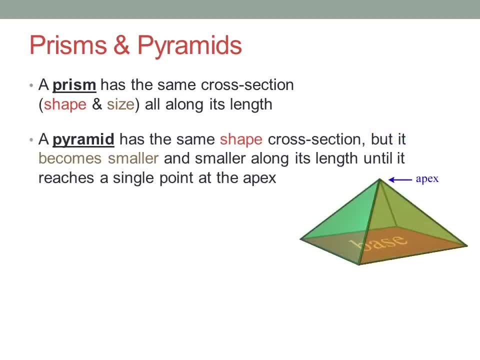 A pyramid, on the other hand, has the same shape- cross-section, but it gradually becomes smaller and smaller until it reaches a single point. That point is called the apex of the pyramid. Again, the base may not always be the one on the bottom. 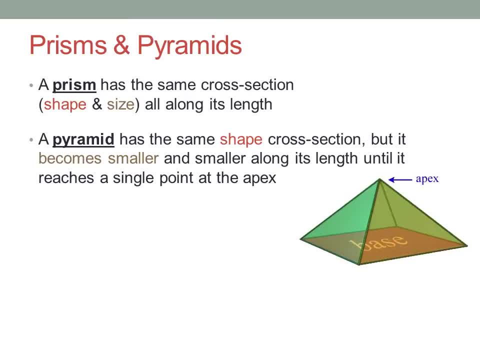 Let's try classifying a few things. Let's start with the base, Let's start with the bottom, Let's start with the top. This is the top edge. The bottom edge is the second biggest point it faces when you look at it. 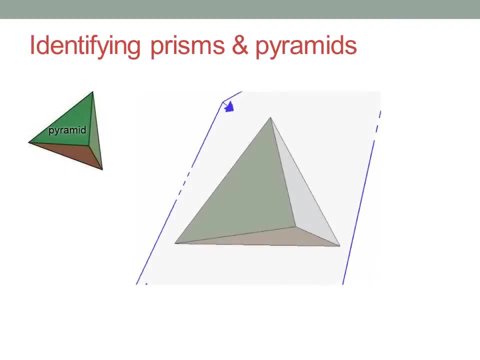 from our perspective, You can see a crack on the top. The bottom edge is the first turning point in the mountain pack. We have a typical pyramid shapes as prisms or pyramids. This tetrahedron is a pyramid because whichever face you choose, 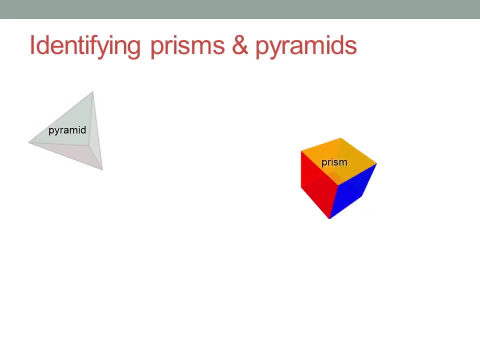 if you take cross sections parallel to that face, you'll get equilateral triangles, like the cross section will stay exactly the same all the way through. It's a square based prism. This one is a triangle based prism, As I showed you just before. you have to be careful to. 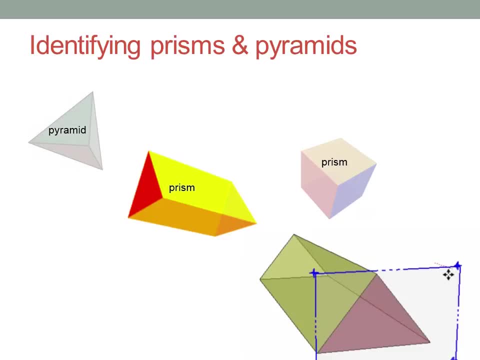 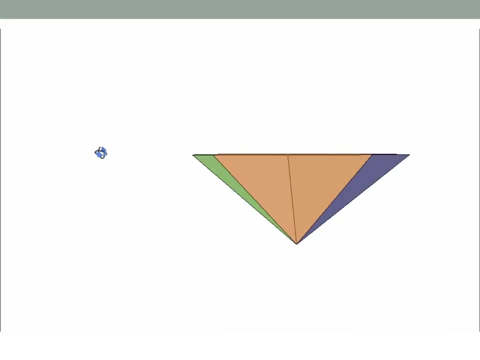 select the correct face as the base. Here you need to choose one of the triangular faces on the ends. Hmm, what about this one? Well, there's quite a few faces meeting at one point. Do you think that might be the apex of a pyramid? Let's try it. Choose the opposite face as the base. 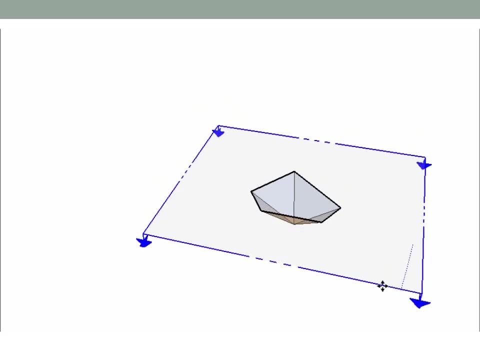 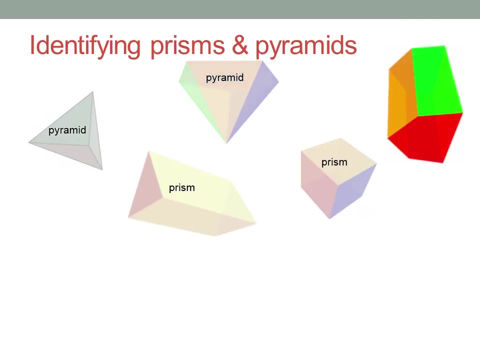 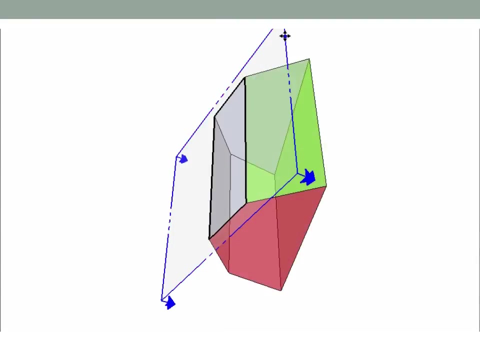 and take cross sections parallel to that base. Yep, the same shape all the way along, tapering to a single point at the apex. It's an irregular pentagon-based pyramid. Can you work this one out? Choose carefully which side should be the base. This side won't. 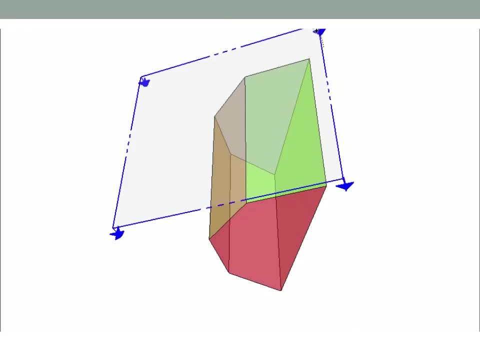 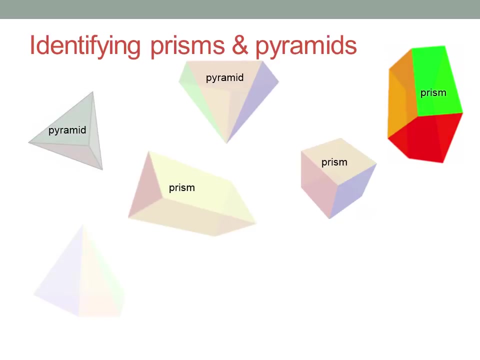 work. Nor will this one. Ah, but this one does. It's an irregular, pentagon-based pyramid. This one should be easier – now you got the idea. Can you see the base? It's getting smaller to a point, so it's a pyramid. 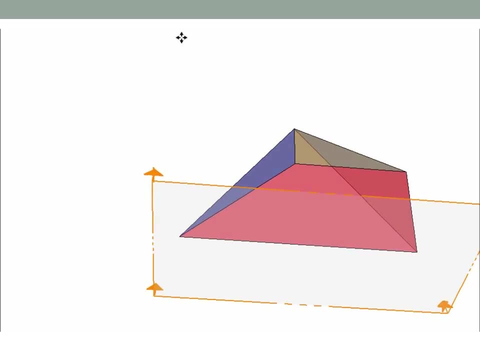 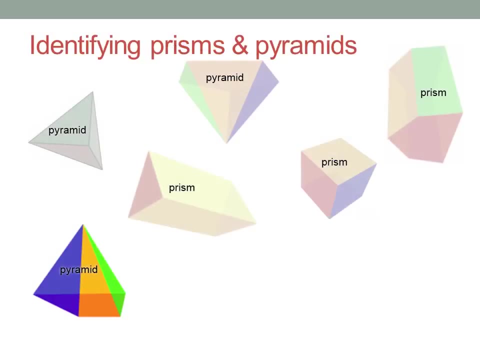 What shape is that cross section? I see two parallel sides. it's a trapezium. This is a trapezium based pyramid. What shape is this? right here Is it rather small. Nom Ça a tropezium. 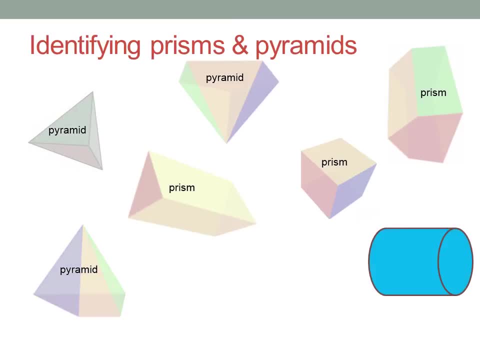 Trans. Regardless what shape is this? parameters is? we still have a pyramid walking知 limits. Now what about a cylinder? Some people say it's not a prism because one of its faces is curved. Well, it's certainly not a polyhedron, because a polyhedron has to have all flat faces. 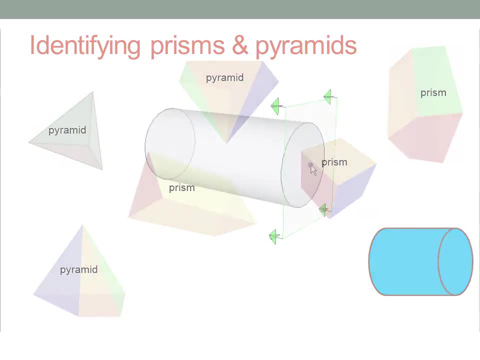 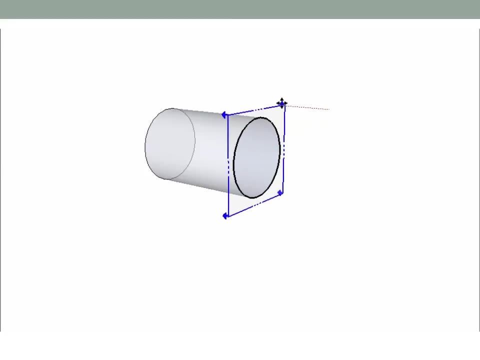 But by our definition a cylinder is a prism. It has a flat base, the circle on the end, and if we look at a cross section parallel to that end, we see the same circle all the way along. That means it's a circle-based prism. 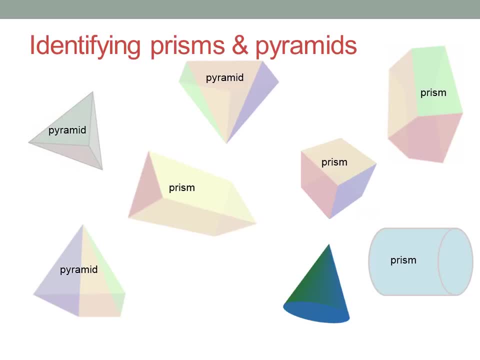 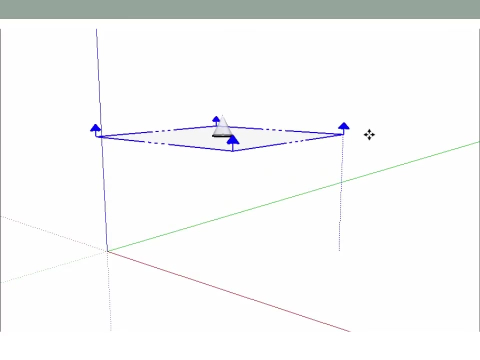 Similarly, a cone is not a polyhedron because it has a curved face, But it is a pyramid. Again, take the circle as the base. There's a circular cross section getting smaller and smaller to a single point at the apex. It's a circle-based pyramid.